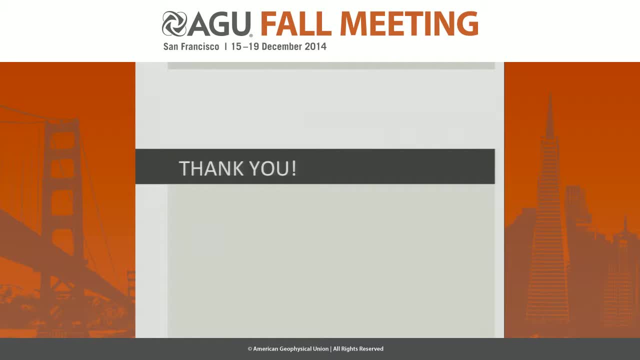 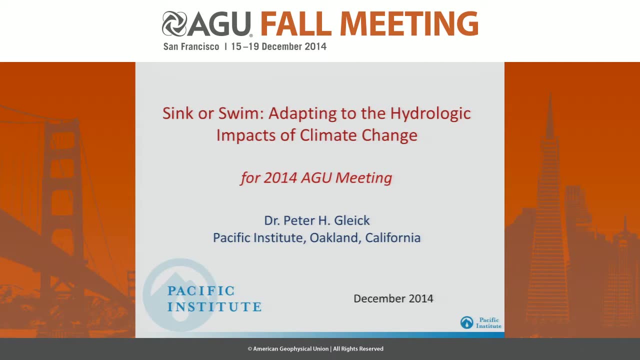 Good afternoon everyone. This is a great session. I want to second Catherine's comments. We heard from Bob about the challenges that policymakers have with communicating risk when they don't understand the biggest risk. I'm going to add the point that managers don't understand those things either. in the context of water resources and, of course, other things That relates to the cognitive issues that Stefan addressed. We work with our existing tools, but that may not be enough And again, in the water area, we're not going to be able to do that. 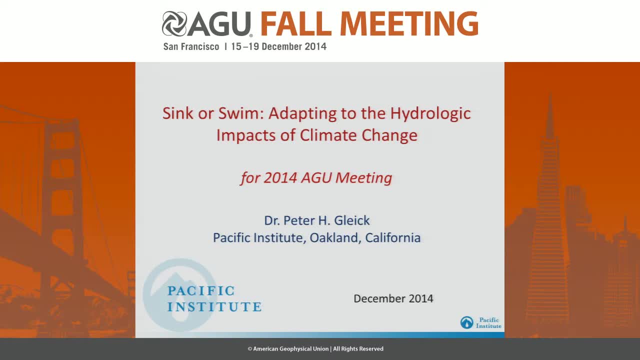 Our managers work with existing tools, but climate change may pose some challenges outside of their experience or outside of the ability of their tools to manage. And Catherine talked about the importance of preparing for these things and raised a question about how and offered some practical thoughts. And if I can get Catherine to come and work with California water managers to solve our water problems, that would be a huge advantage. Let me just leave that at that. 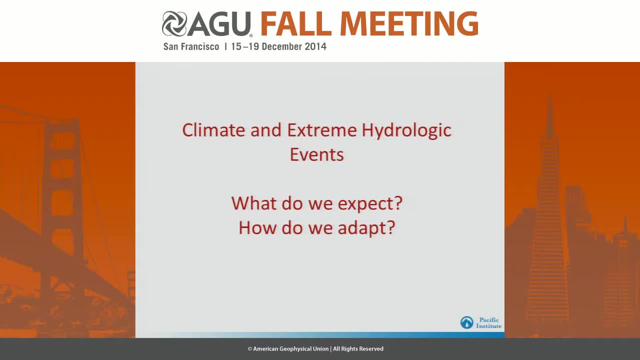 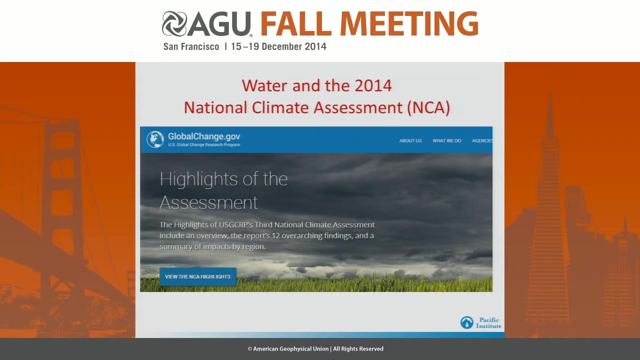 Okay, So I'm going to talk about climate change and extreme hydrologic events. I'm going to talk a little bit about the science, of what we know, what we expect and what we see, and then a little bit about the policy, about how we might want to adapt. Some of this is going to come from the National Climate Assessment that was mentioned earlier, some work that we've been doing, some global work from the IPCC on extreme hydrologic events. 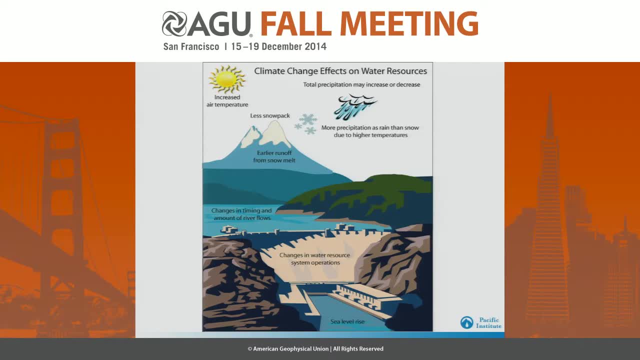 I like to talk about water in the context of climate change, in part because I'm a water guy, But also in part because the hydrologic cycle is the climate cycle. As we change the climate, we're going to affect pretty much every aspect of the hydrologic cycle, from the natural perspective, but also from the perspective of the infrastructure that we build: the hydrologic, the dams that we build to store wet years so that we can use it in dry years, the infrastructure we build for water treatment and management, And I'm going to make some comments about some of the infrastructure issues as well. 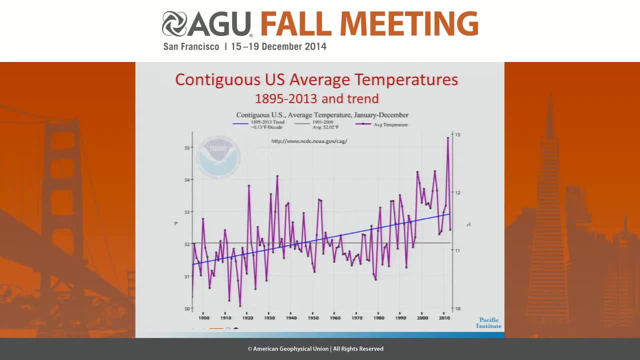 This is a graph that shows contiguous US average temperatures over time over the last hundred. and what is it- 118 years or so- showing the trend in temperatures in the US. We saw some of this locally already. Already we know the news is coming out that this may be the hottest year on record globally. It's, without a doubt, going to be the hottest year on record in California in the 2014 timeframe. 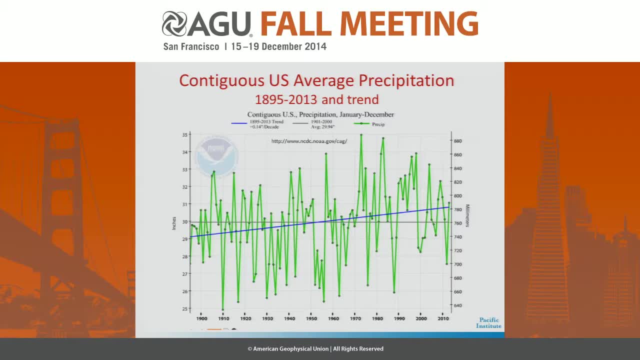 But we also see these changes in predictability And we're also seeing changes in precipitation trends And again Catherine showed a graph I'm going to show also for changes in precipitation patterns in the US. This is the same trend for the continental United States. 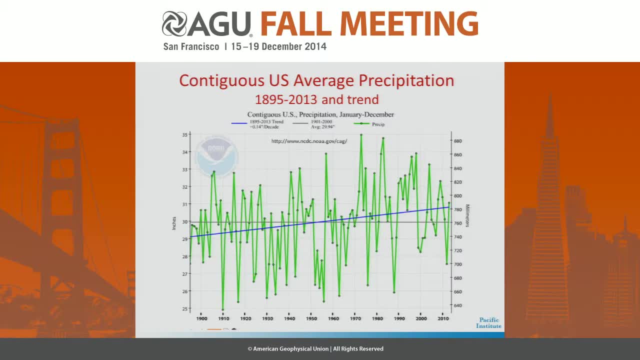 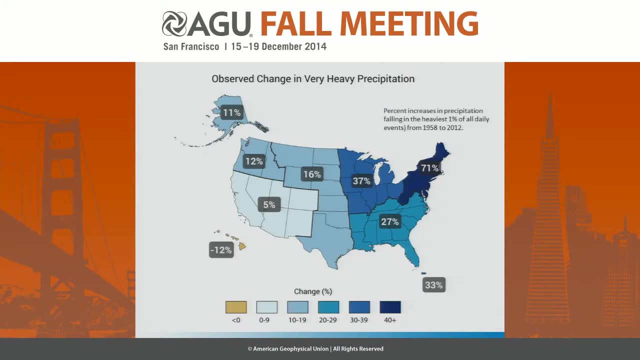 We know that a hotter planet means more evaporation, more moisture in the atmosphere. The observations suggest that, Theories suggest that, Models suggest that, And that's the way we're moving. This is the graph that Catherine showed, showing we're already observing changes in extreme precipitation events in the United States. 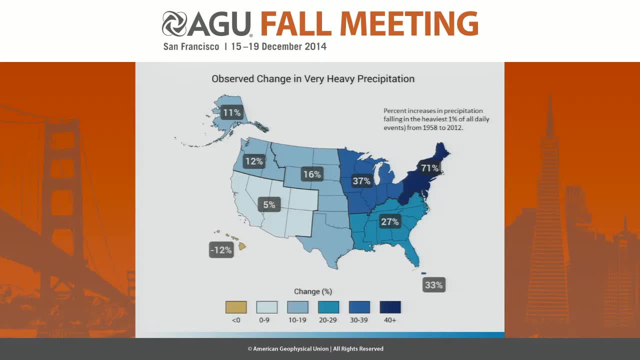 Something that we're already observing, And we're already observing changes in extreme precipitation events in the United States, Something that we're already observing. This was projected many years ago by theory, projected by model output as well, And now we're seeing in observations. This shows basically the percent increases in precipitation falling in the heaviest 1% of daily events over the last four or five or six decades. 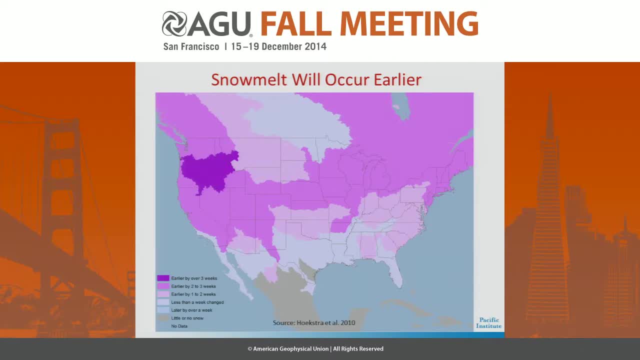 We know that one of the things that's going to occur, and is already occurring, is changes in snowfall and snowmelt dynamics. Some of this was the work I did years ago in California. Higher temperatures, even if there's no particular change in precipitation, means more rain and less snow. 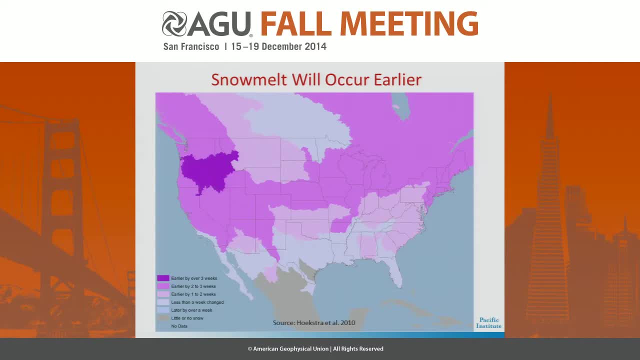 In the Sierra Nevada, in the Rocky Mountains. it means what does fall is snow melts faster and runs off earlier, So we see a change in the timing of runoff. So snowmelt dynamics is going to be an important part of water management challenges for policymakers and water managers. 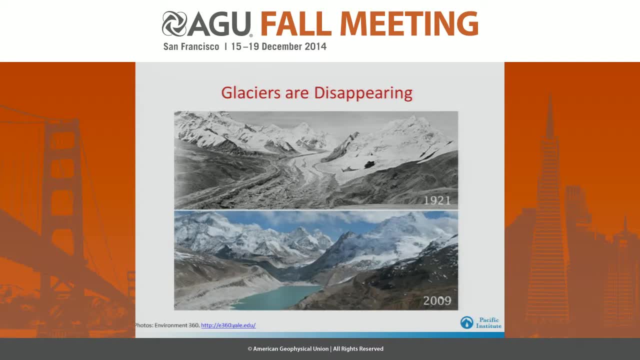 We know the glaciers are disappearing. This is going to be an issue not just for natural ecosystems, but for downstream water infrastructure and populations that live downstream. There's been a lot of discussion about this in the context of the Himalayas, but it's true for other parts of the world as well. 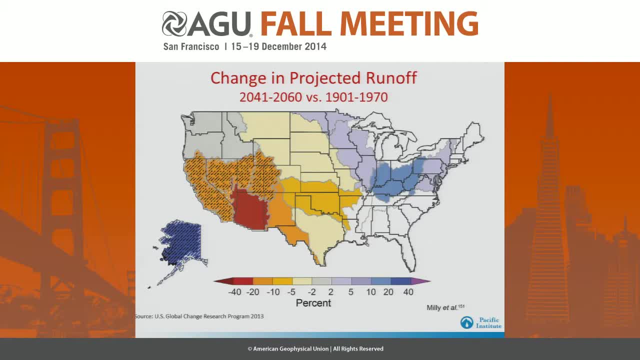 There's been some estimates of changes in runoff And, ironically and unfortunately, some of the most significant decreases in projected runoff are in those regions, in this case of the United States, that we already know. Some of those regions that we know are warm and dry, where there are water shortages and competition over water resources. 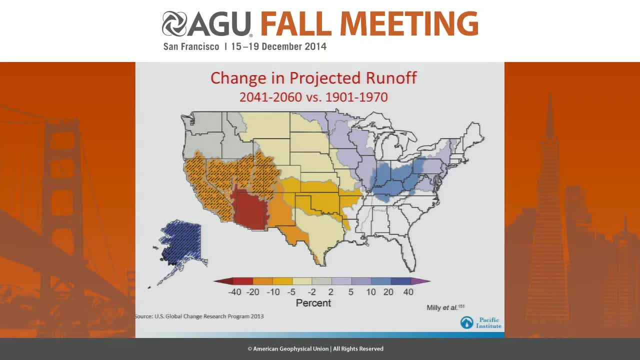 This shows basically very significant projected decreases in runoff in the Colorado River Basin in particular and the southwestern United States in general, And for some of these basins these are already over-allocated basins. These are basins even without climate change. we have very serious water management problems. 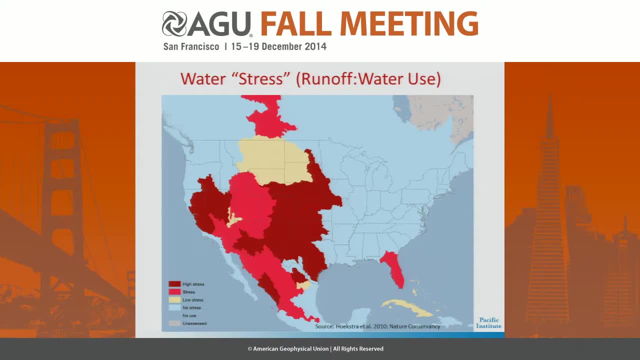 And when you impose climate change on these challenges, it makes current difficulties even worse. When you put these things together, you get water stress of different kinds. There are lots of different indices out there that people use to measure water stress. This is one that compares the amount of runoff versus the amount of water demanded or used in a region. when you put together all of those factors, 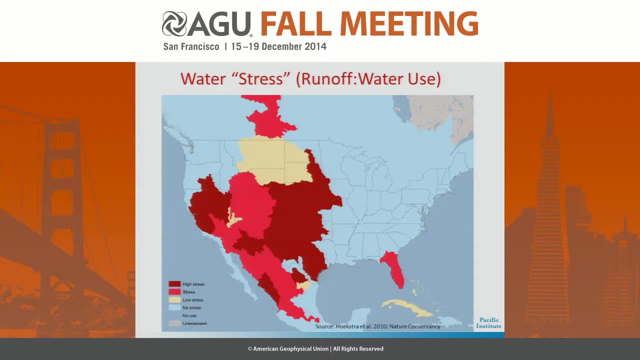 And again it shows what we already know from models. We already know from model projections and from existing challenges, which is that the warm, dry, arid west is a place where we're going to have serious problems. But I want to talk about some things that we don't tend to think about. 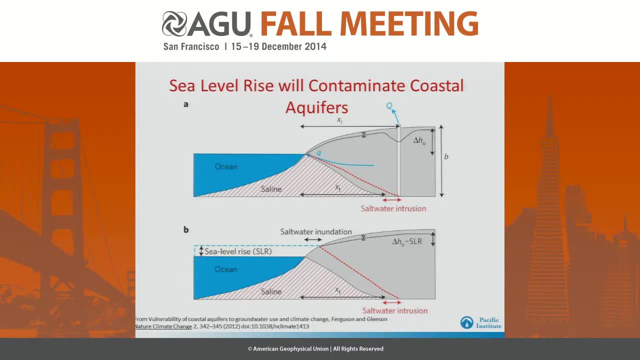 We think about water availability, We think about stress, We think about changes in runoff, But water is a big issue. Another piece of this puzzle is the issue of sea level rise. It turns out that sea level rise can have impacts on coastal ecosystems where fresh water and salt water mix. 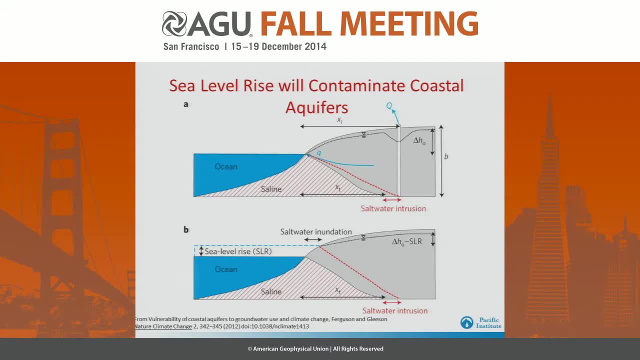 So we're going to talk about that in just a moment. So aquatic and salt and freshwater ecosystems are going to be affected by sea level rise. That's a water challenge in many ways. We draw water from coastal aquifers And as sea levels go up, we're going to see more penetration of salinity into coastal aquifers, even when we're not overdrafting those aquifers, which, unfortunately, we are. 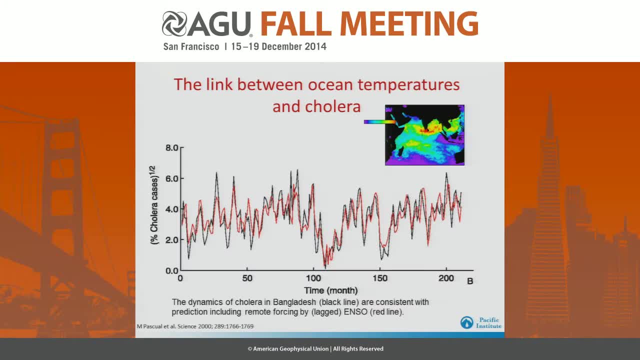 So sea level rise is a freshwater challenge for many communities as well, And there are other issues. There's a very strong connection, it turns out, between sea surface temperature and cholera in the Sea of Bengal and in western Bengal and in India. 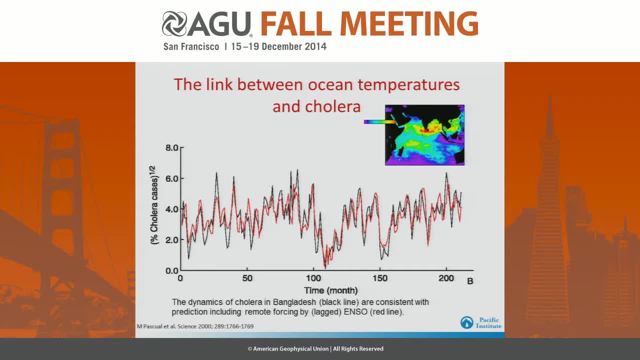 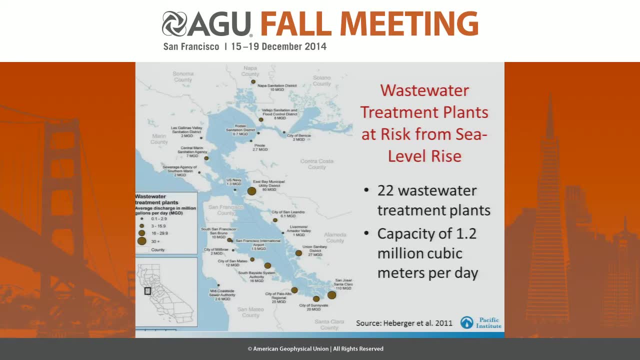 So connections between temperature, connections between sea surface temperatures, connections with public health, especially water-related diseases, are relevant. Here's another one. We did a study at the Pacific Institute a few years ago doing high-resolution mapping of the coast of California. 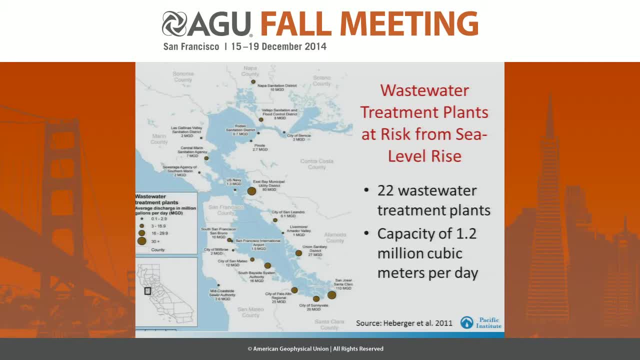 From the Oregon border down to the Mexican border, looking at the implications for infrastructure, populations at risk and so on. And one of the things that people don't tend to think about much, but is apparently a special vulnerability, is wastewater treatment plants. We build our wastewater treatment plants at the coast because what we do is we collect wastewater, we treat it to some standard and then we throw it away by typically dumping it in the ocean. 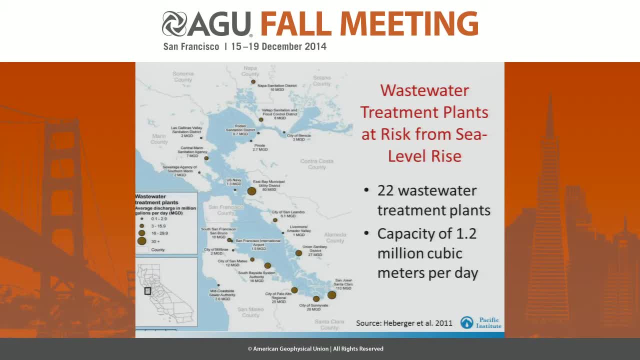 That's a water policy issue. I won't get into the details. It's a very interesting questions about reusing wastewater in California. There are some wonderful policy challenges there, But it turns out for the Bay Area alone there are 22 wastewater treatment plants within a meter of sea level rise that are vulnerable to the sea level rises we expect over the coming decades. that will either have to be protected by building sea walls. 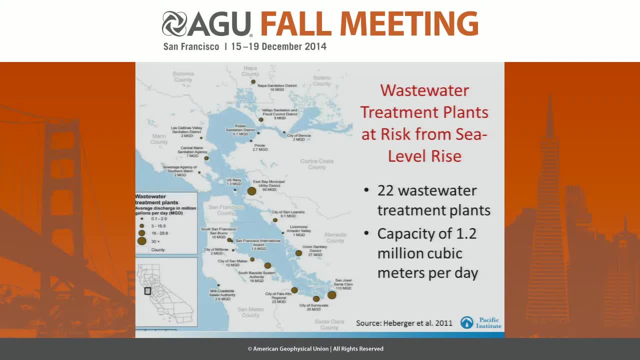 They'll have to be modified by raising outflow structures. They'll have to be abandoned and moved if the costs, Depending on the climate, Right. That's one of the options that are available to water managers, And it's safe to say that water managers aren't thinking about this now. 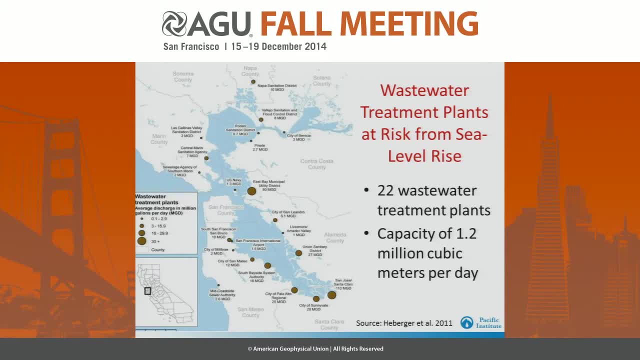 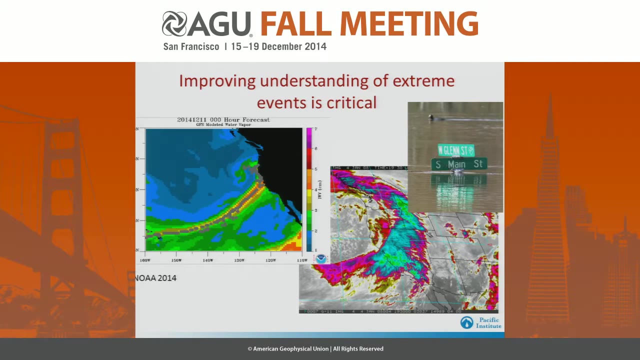 And maybe in Katherine's, from Katherine's example. explaining these kinds of challenges and threats to water managers helps raise issues that might they might not otherwise be thinking about. Broadly speaking, we worry about extreme events, Obviously. we worry about averages. 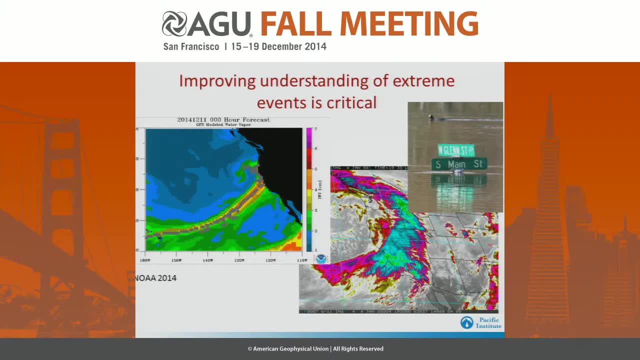 But again from Steven's talk, we worry especially about extreme events. We don't fully understand The implications of extreme events. The picture on the left is from a couple of weeks ago. It's the atmospheric river that dumped a huge amount of rainfall on northern California. 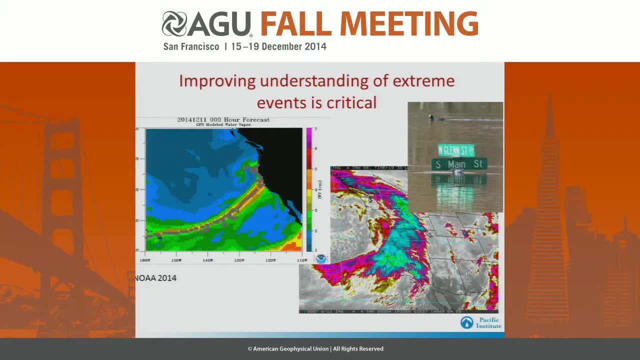 This was the sink or swim event that Jim mentioned a moment ago when he arrived at the airport. We get our precipitation on the western, in the western United States, not in slow, occasional rainfalls, but in extreme events, And we don't fully understand what climate change is going to do. 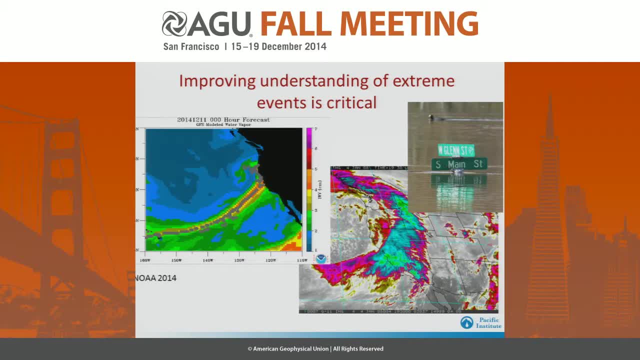 We don't fully understand what climate change is going to do to those extreme events, Although, what I would note, in the last few years there's been a tremendous increase and a number of very interesting papers looking at changes in sea surface temperature, looking at changes in atmospheric dynamics and pressure systems off the Arctic. 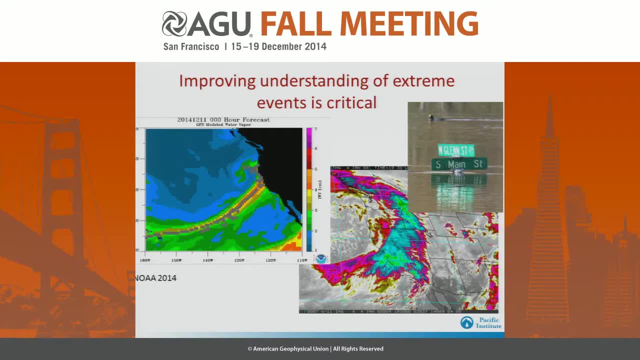 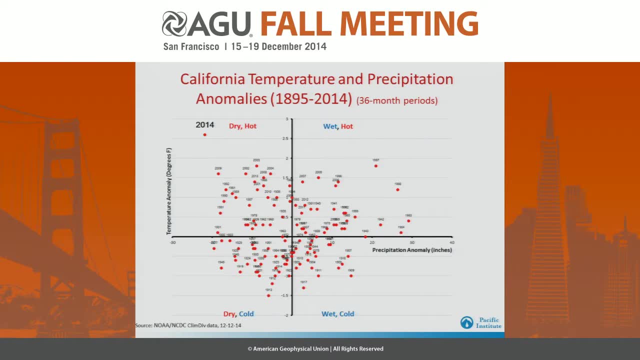 And the implications of those kinds of changes for water resources in the western United States and in California in particular. One comment about the drought For those of you who don't know The drought. for those of you who saw my talk on Tuesday, this is the one slide that you saw. 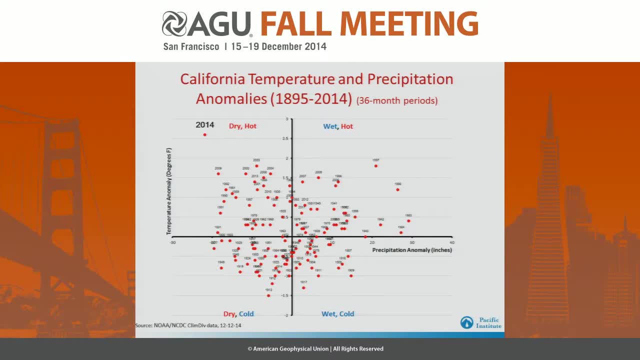 This is California temperature and precipitation anomalies in terms of 36-month three-year averages for every year going back 119 years. Basically, anything that's above the center line, anything above this line here is a warm anomaly, a warm year out of the last 119 years. 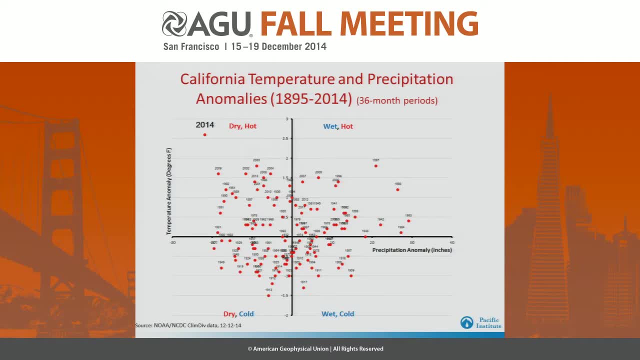 Anything below is a cool year. Anything to the right here is a wet year compared to the average. Anything to the left is a dry year, And each of the last 119 years of our instrumental record are plotted as a point here, And this is 2014.. 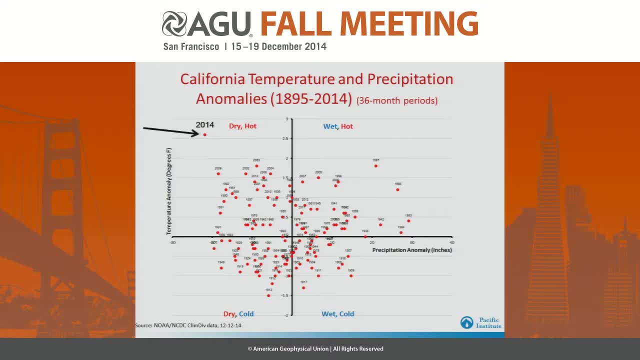 To describe it as an outlier is an understatement. We're in the midst of a three-year drought, Notwithstanding the incredible rains we've had in the last few weeks. Interestingly enough, you can't read the years for most of these, but the hot, dry years are up here and they're the last few decades. 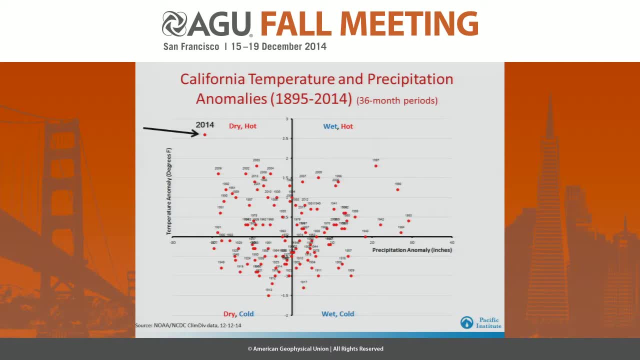 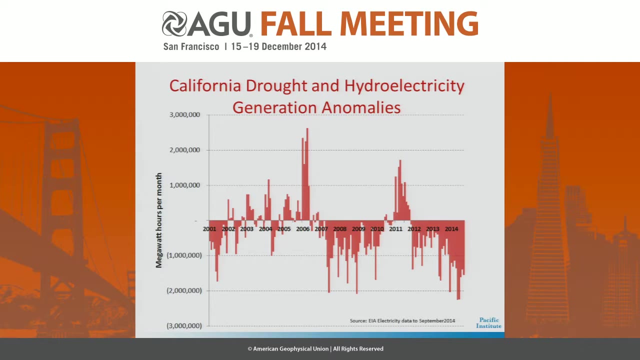 And that's another challenge that we face in thinking about not just drought- We get droughts naturally and floods naturally- but the implications of climate change for those extremes. And then here's another thing that we don't tend to think about. This is work that we're doing at the Pacific Institute. 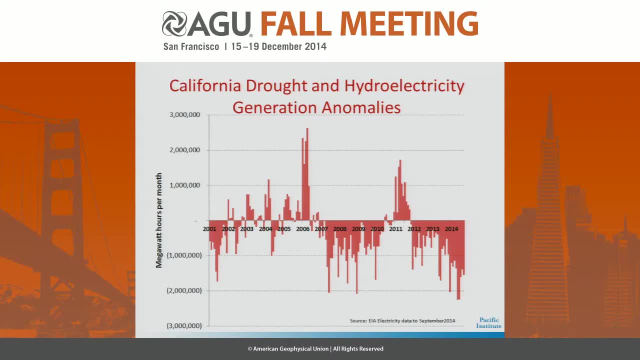 It hasn't yet been released. This is basically hydroelectric generation anomalies over just the last decade or so, about 15 years, and in the context of increases or decreases in monthly hydro generation from the expected average hydro generation for those months. What we basically see here, here especially, is the last three years of drought in California. 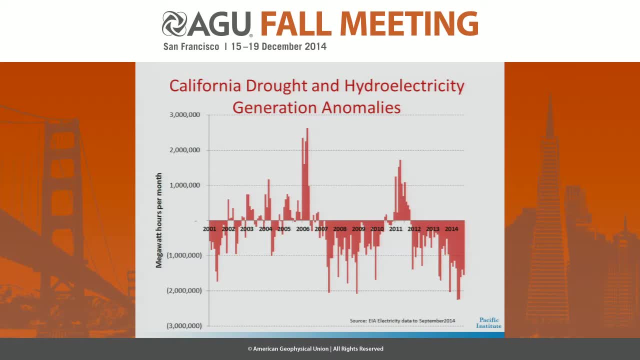 showing that one of the impacts of drought in California is a reduction in hydroelectricity generation. We get less precipitation, less rain and snow. We get less runoff. Our reservoirs are drawn down. We get less hydro generation. Now, in fact, it's not just a three-year drought. 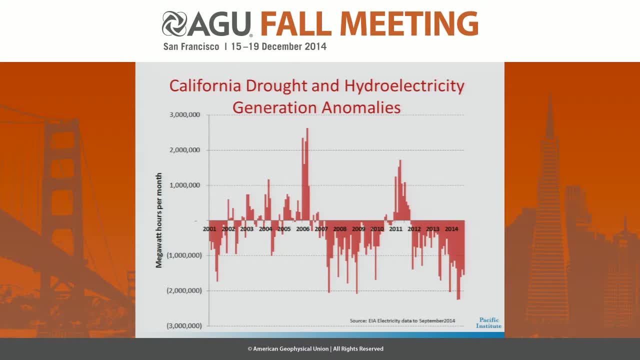 Ten of the last 14 years in California have been dry and there's been a shortfall in hydro generation. What do we do when we get a shortfall in hydro generation? We burn more natural gas. So there's a climate feedback. There's a climate feedback issue associated with that. In addition, consumers pay more money. Hydro generation is relatively cheap. in California We burn more natural gas. It's more expensive. Consumer rates go up. At the moment, our expectation is just over the last three years, this anomalous drop, this drought-driven drop in hydro generation. 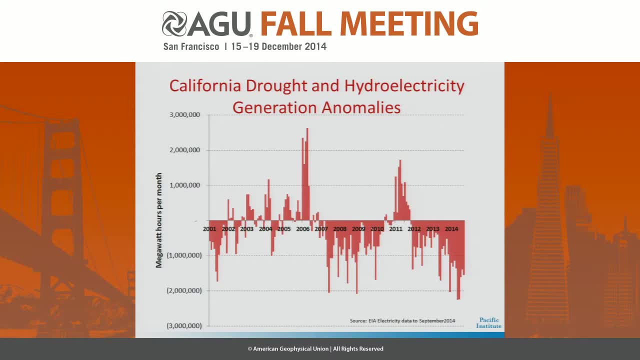 has cost California ratepayers about $2 billion. That's an impact of drought. It's an impact potentially. It's an impact potentially of long-term changes in climate, if that's going to affect hydro generation. So that's something else we have to think about. 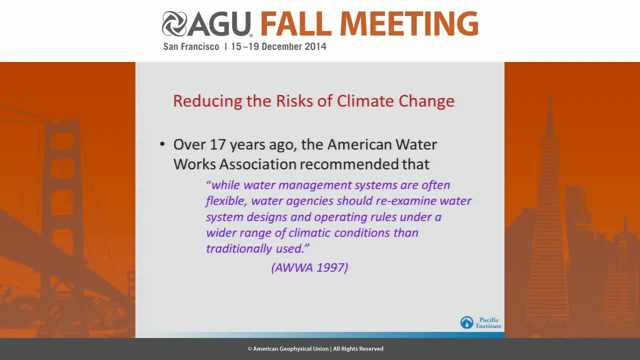 So for the last couple of slides, let me just talk about policy a little bit and the connection between extreme hydrologic events and policy, And I would argue this is not a new issue. I was on a panel with the American Water Works Association 17 years ago or so in which 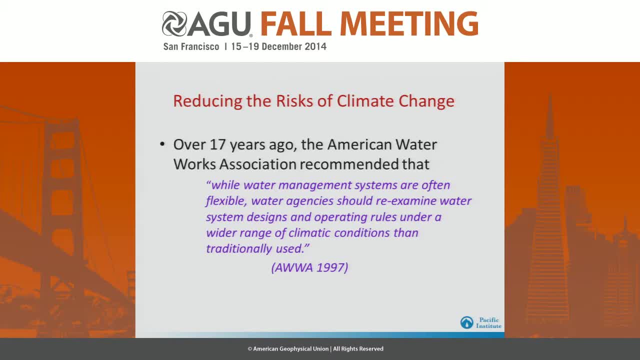 and the American Water Works Association is basically an association of 50, 50,000, 56,000 water utilities around the country, And they concluded then, almost two decades ago, that, while water management systems are often flexible, water agencies should reexamine water systems design and operating rules under a wider range. 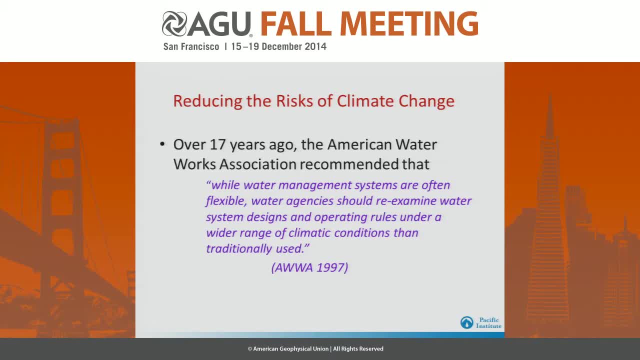 of climate conditions than traditionally used, And it's the point that was made by earlier speakers. Our system is designed on the assumption, our infrastructure is built on the assumption that tomorrow's climate is going to look like yesterday, Yesterday's climate And, if there's anything that we know, despite the uncertainties about precision predictions, 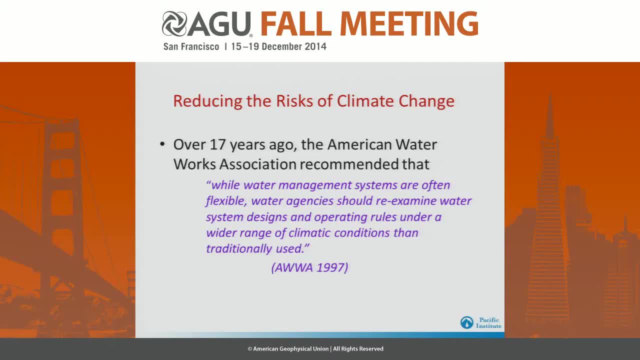 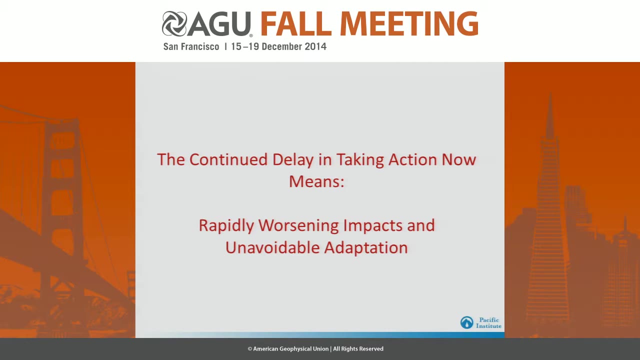 for the next 20 years. it's that that assumption is wrong. It's that the climate's changing and we had better rethink our management strategies under a broader range of scenarios, And yet we're still not doing that today. So the longer we delay in taking action, the worse will be the impacts. 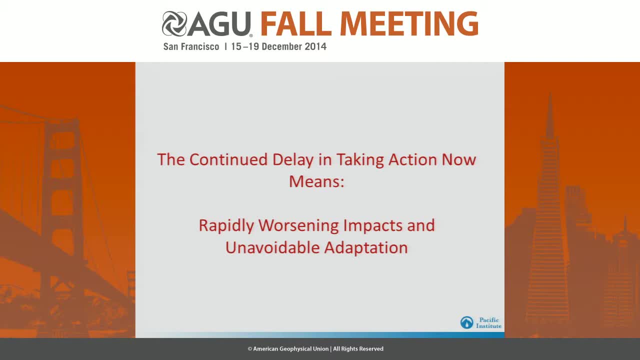 and the greater will be the levels of adaptation That we have to pursue. and I'm not going to get into the debate about mitigation versus adaptation. I think it's pretty obvious we have to do both. But let me just close with some comments about strategies. 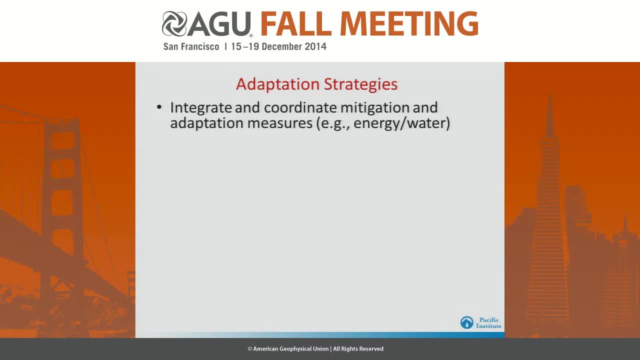 We have to integrate and coordinate mitigation and adaptation. There are strategies that we can pursue on our energy system and our water system that helps us adapt to unavoidable impacts and yet may help us mitigate the emissions of greenhouse gases. and the example I just gave about hydroelectricity, where reductions in hydropower mean burning more natural gas.